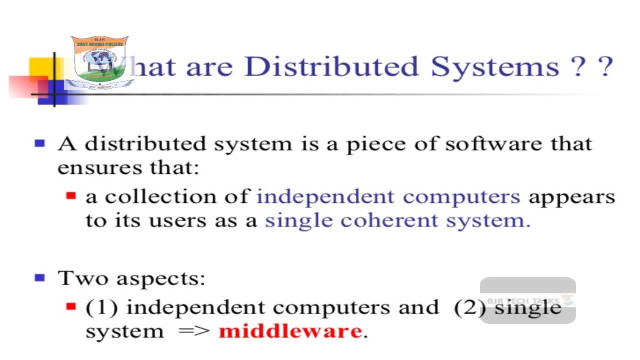 since they came, or they are working as a team or a group, so you can say that the system, the whole system, is a distributed system. So let us try to understand the basic definition again. What is the basic definition? A distributed system is a collection of physically separate. that means the. 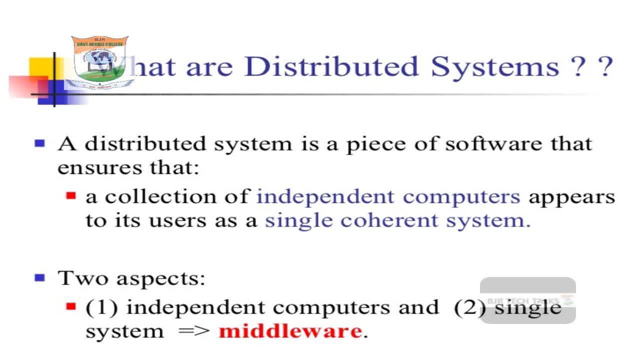 systems are not physically near, they are separated. so a distributed system is a collection of physically separate and possibly heterogeneous. So all these systems are of not same kind. One might be a supercomputer, or one might be a workstation, one might be a desktop computer. assume like that. 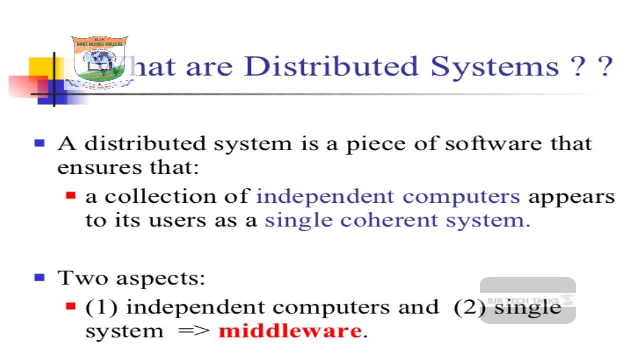 so all these have different processing speeds and different mechanisms right at the same time, so you can say that the distributed systems are physically separate. i mean, it's a collection of systems which are physically separate and possibly they might work with the heterogeneous data, and so how they're going to be connected? yeah, using some kind of network, these systems have been. 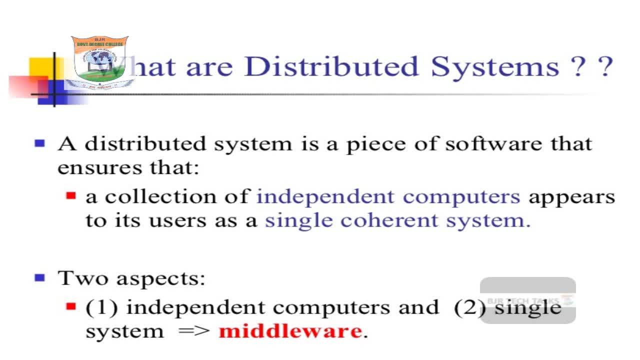 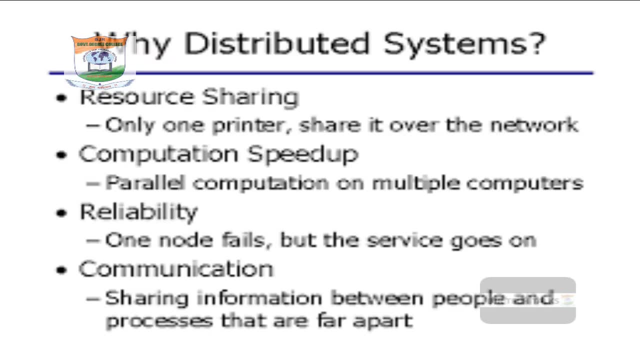 interconnected. what is the main purpose for them? the main purpose for them is to provide the users with access to various resources. that's the main purpose. so, even though these systems have been located different locations, the main purpose is their form as a group and they try to 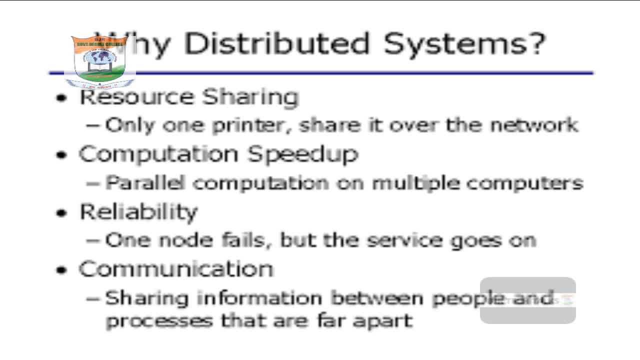 serve the user with the data and the resources. so what does it mean? for example, if you have a resource which is a shared resource, assume, like that, i have a resource and i say that there is a shared resource. so what happens if you have the shared resource, automatically it is going to be. 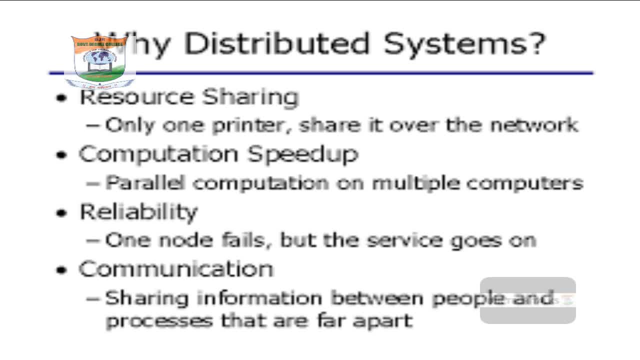 increasing the computation speed, functionality, data availability and reliability. that is the basic advantage of distributed systems. what does it mean so? what does it mean, for example, you have a shared work or a shared resource, instead of purchasing different resources. if you have only one resource, for example, i say there is a server, assume like that there is a server which can do. 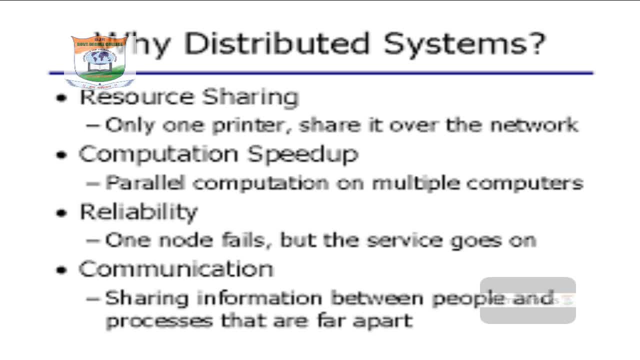 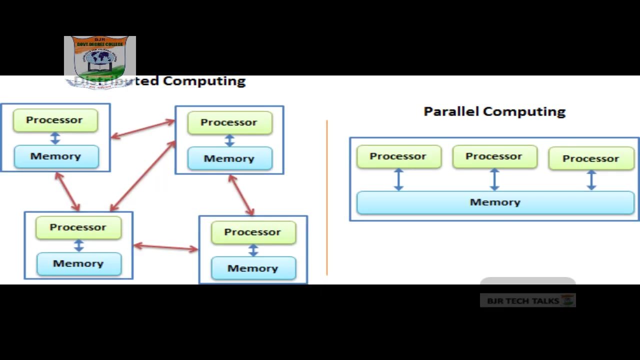 use computation. there is a server which can do use computation. okay, right, and if all the systems which are located in the distributed system, or if all the systems which are located in the group remotely can take the services of that server, then then you can assume, then you can achieve increased computation, you can achieve good functionality, data availability. 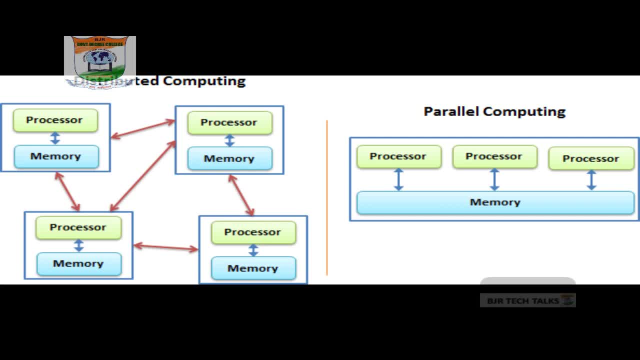 and reliability. instead of purchasing various data servers, why don't you go for minimal amount of data servers, kept them available to the systems and made use of that? this is the basic advantage of distributed system. see, the same thing happens with the google, yahoo, etc. you've been accessing the google data right? google has kept different. 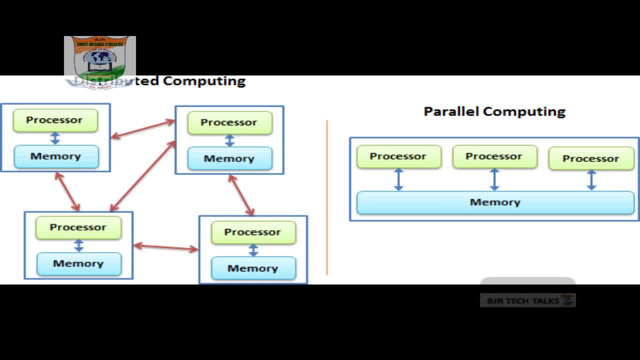 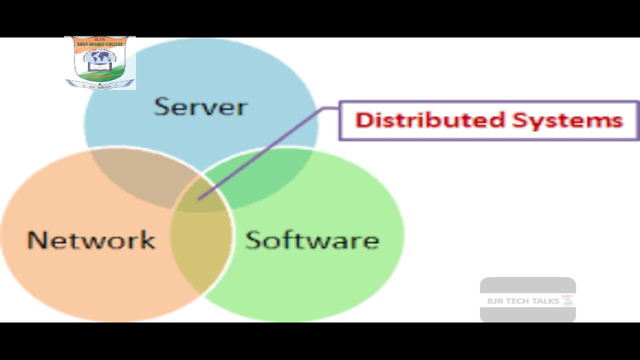 servers at different locations. okay, then what happens? okay, your request will be redirect to one server and you don't know where the server is located. and you don't know where the server is located, but the server is trying to. but the server is trying to provide the data at the same time time. 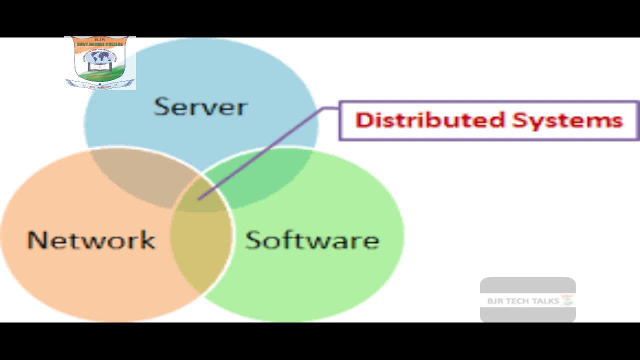 server is trying to help your request. so this is the basic concept, or basic underlying concept with the distributed systems. so what is the basic property here? here, the resources are shared. okay, so what is the advantage of sharing a resource, right, if you have a resource which is shared? 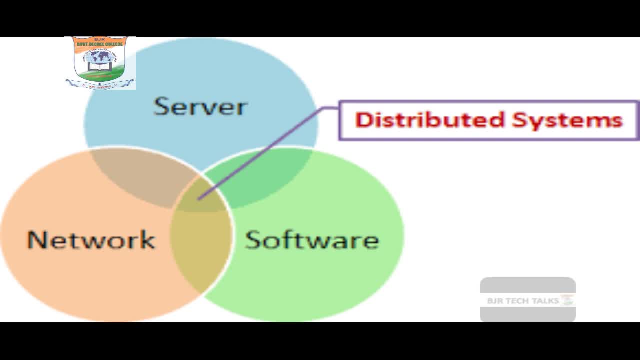 then it compute, mean it increases the computation speed, functionality, data availability and reliability. so these are the basic advantages. if you try to put a resource as a shader resource- and this is the basic property of the distributed system- see distributed system- is the is also called, as we have already previously discussed, but let me try to remind you the loosely coupled system, the, 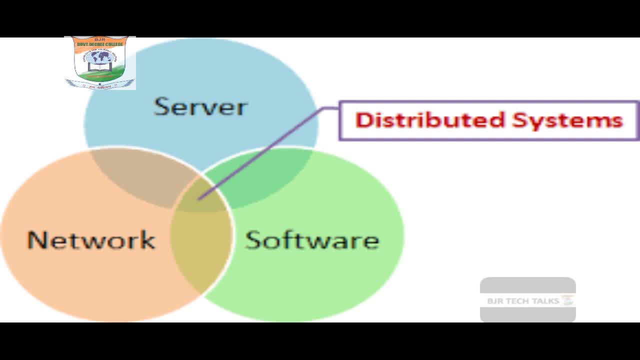 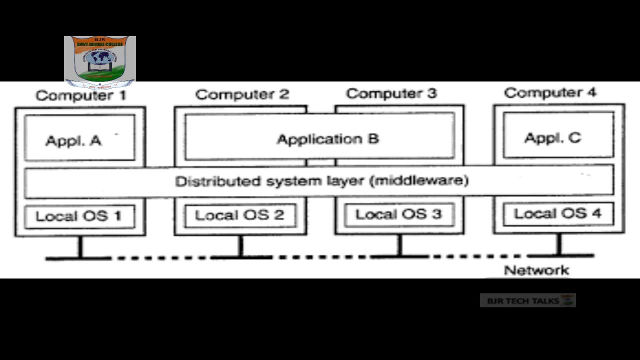 a newly coupled system is also called as the distributed system. very simple, the name itself is having the distributed, so everything has been distributed at different locations and you're simply accessing them whenever you're they're needed. there is a basic advantage. now we will put a question: how this distributedness can be achieved. it's very simple: you have a separate 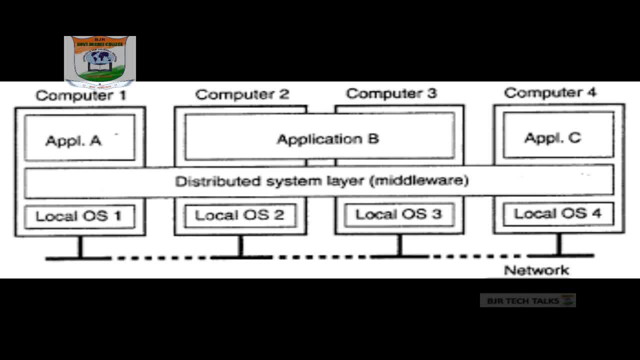 software for separate operating systems that can support the intelligence that is required for a this distributed property. so a traditional operating system will not support that. but anyway, distributed systems have their own operating system. so some operating systems, something like, they generalize network access in the form of file access. see what happens. 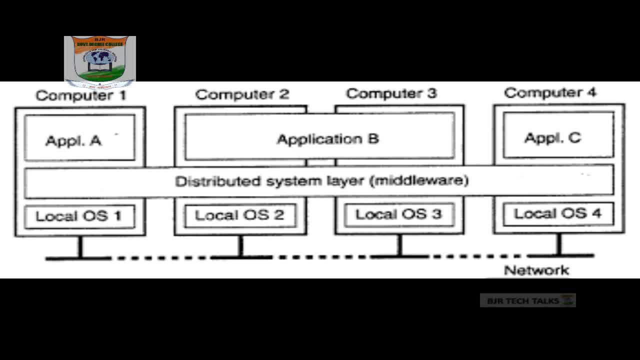 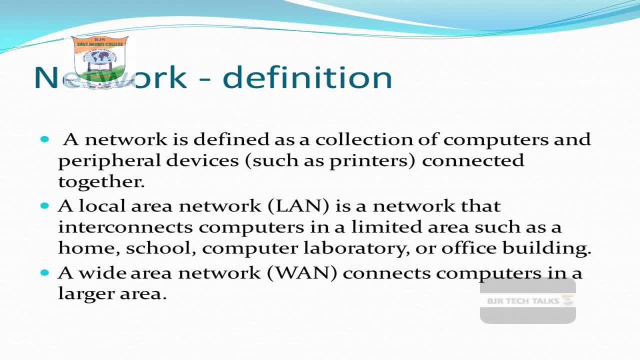 with the details of networking contained the in the networking device drivers. let us try to know some simple terminology regarding the distributed system. the first terminology is a network. so what do you mean by network? so I can say that a network in simple terms, I can say that a network is a communication path between two or more systems. 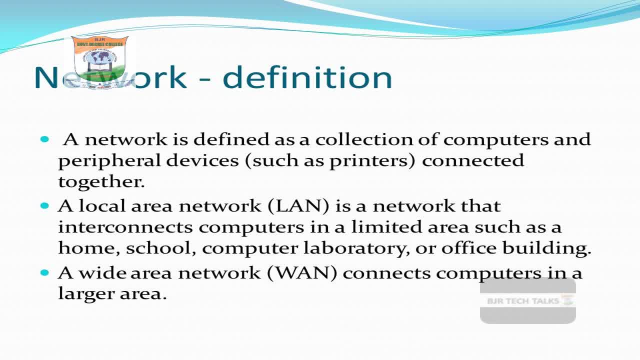 that's it. so you have two or more systems, whether it is a phone, it is a computer, desktop, a workstation or any super computer, anything. you have two or more devices and assume that if you try to interconnect them, then call it as a network, correct or not right? so distributed systems depend on networking. so if you don't, 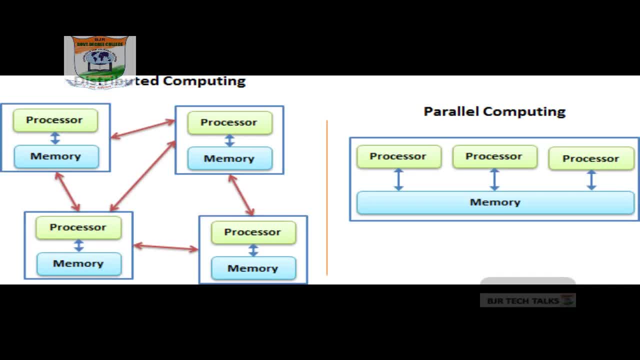 have network, assume there is no distributed system. the basic requirement for the distributed systems is that all the systems are, should be, connected through a network. if there is no network, then you cannot create a distributed system and these networks vary or differentiate with the protocols they work with. see these networks. 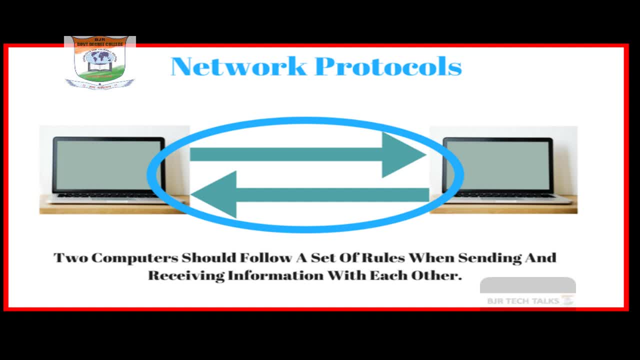 have different protocols and one system may work with one protocol, another system may work with another protocol. I mean they have their own mechanisms. protocol means set of rules for working right. so assume that all the systems, even though they work in the network, these systems work in a network or these networks will have different protocols or different set of rules to work. 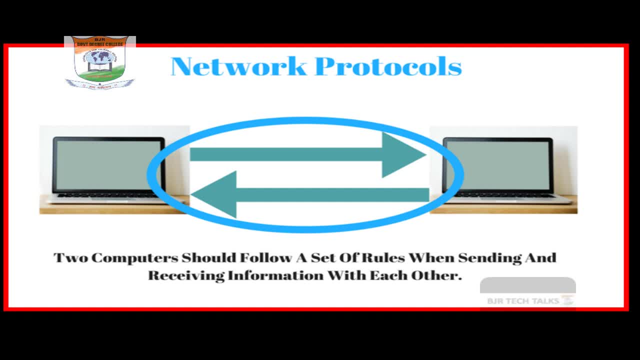 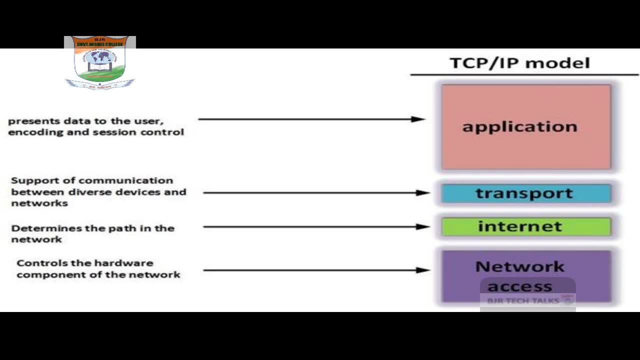 with and my dear friends, TCP IP, TCP IP, TCP IP. so TCP IP is the most common network protocol. you have to remember this point. okay, TCP IP is the most common network protocol. we'll try to understand more about this in the next sections, but anyway, try to remember this point. 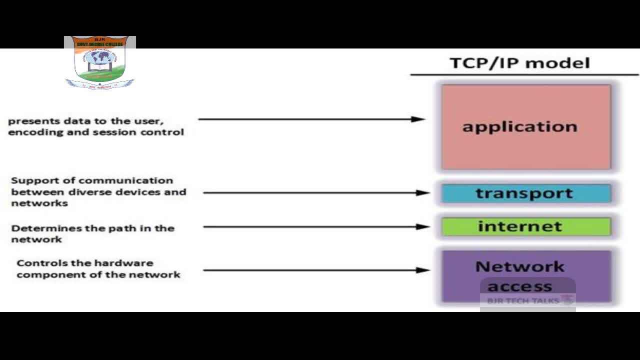 okay that TCP IP is the one of the most common network protocol and TCP IP means transmission control program or protocol and internet protocol. The name itself is that. So transmission and control protocol slash means it is also having an internet protocol. This is the core protocols in that. 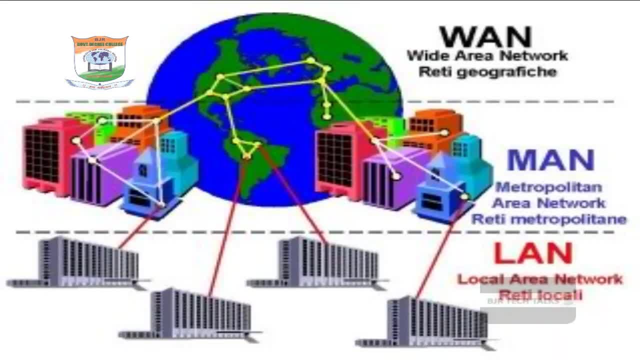 networking layer. right, Again, we have three kinds of networks. Again we have three kinds of networks. The first network is the local area. network means if you, if you have constructed a network, I mean an interconnection between the systems and which are confined within a small 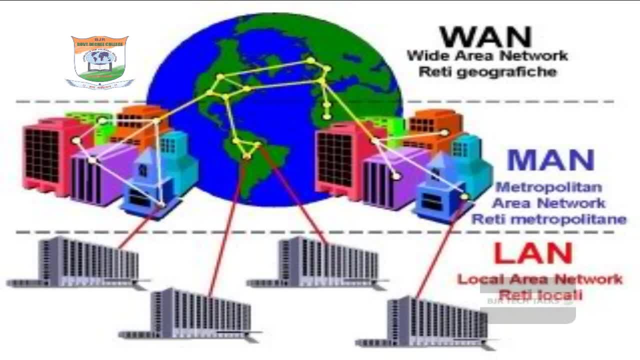 meters, probably within, confined within a building or within a campus, then call it as a local area network. And if your network, if your network, is confined within a particular system, city or area, then you call it as a metropolitan area network. This is second kind And third. 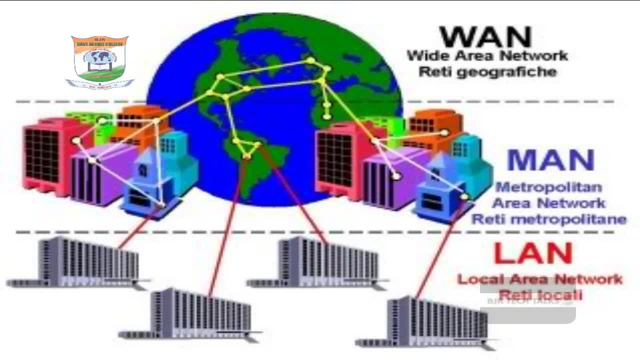 kind is if the network is spread or distributed across a vast area or over the globe, then call it as the wide area network. So that means the internet capital I, the internet right now we are using, is an example for the wide area network And the network or the network is. 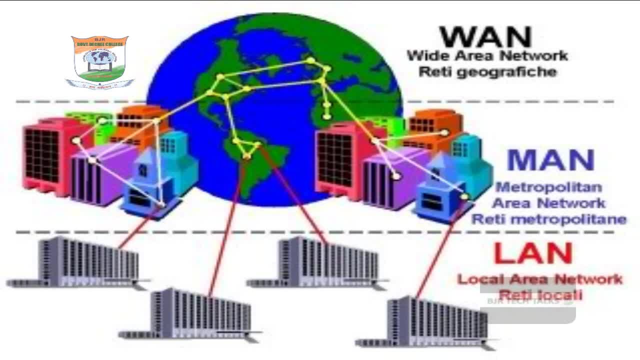 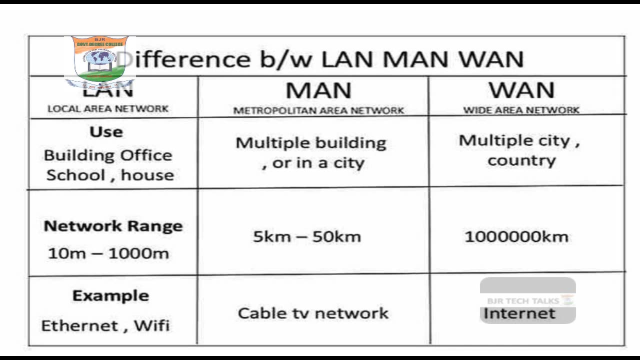 for the computer network which you have in your college lab or in your office campus, then call it as the local area network And the broadband network which is provided for you in your city. That is an example for the metropolitan area network, also called as the man, So for the local area. 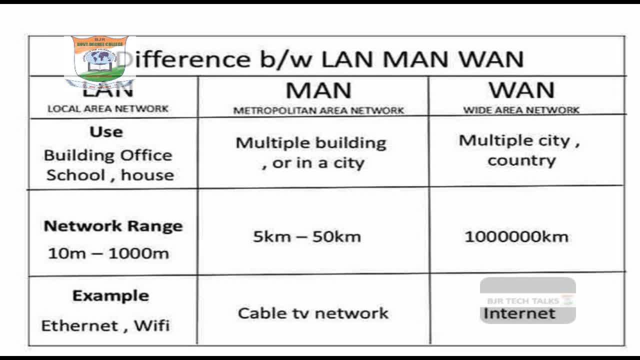 network called as the LAN, and for the metropolitan area network called as the MAN, and third kind wide area network also called as van. okay, so if it is confined within an office or an institute or it's a campus extending few meters, call it as the land if it is geographically completely distributed. 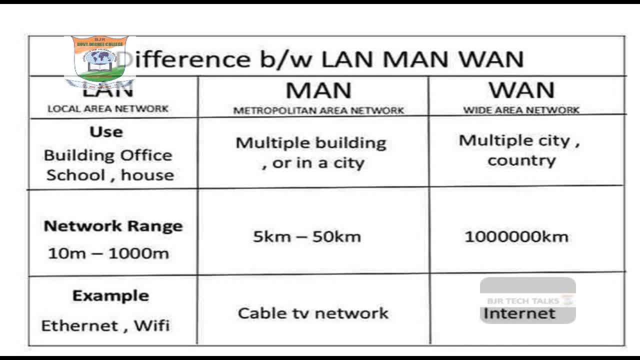 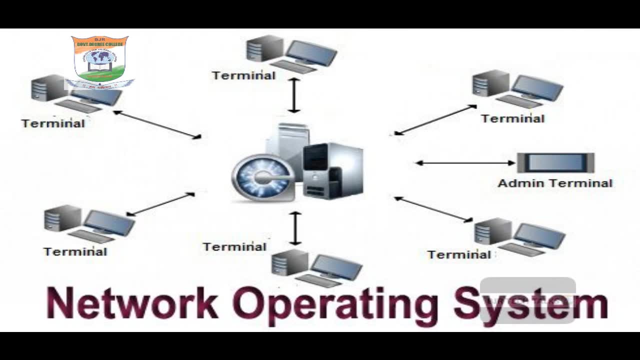 call it as the van if it is confined to a city limits. call it as the man see. let us try to understand what is the speciality with these operating system. when you work with a network, see the operating system. okay, the operating system which supports a network, the operating system which supports a network, is called a network operating system. 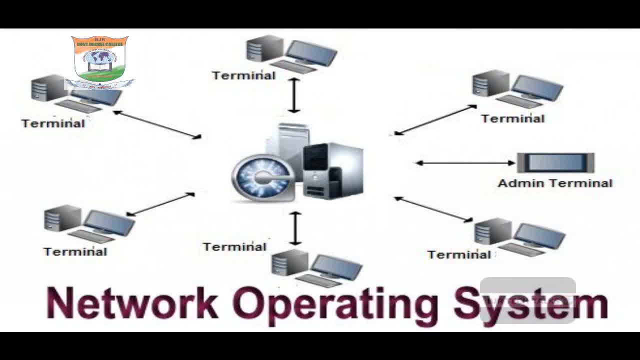 a operating system which supports a network is called a network operating system, and this operating system is going to provide certain features like file sharing across the network and also includes a communication scheme. so this network operating system is not a traditional operating system, rather it is having, as it is providing, special 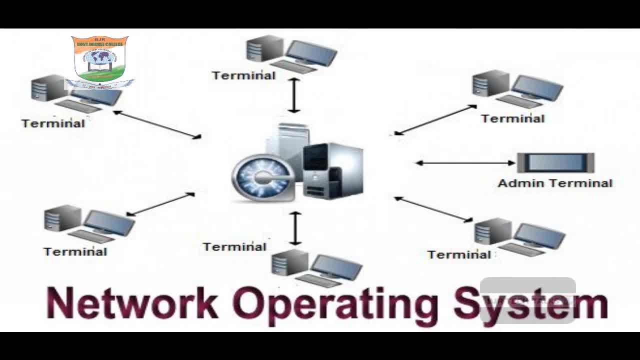 features like file sharing across the across the network. so you have different systems and this network operating system is going to help you to share the files across the network and also and also includes a communication scheme in such a way that in such a way that different computers can exchange messages. so the process: 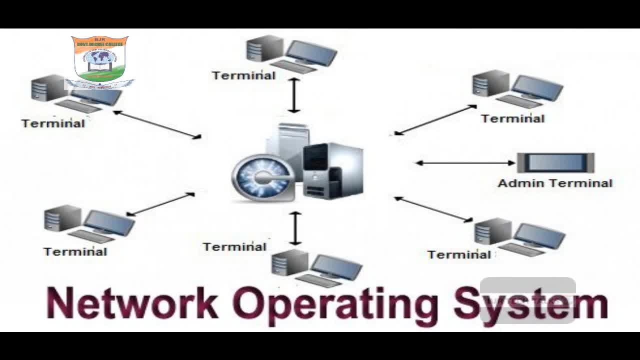 at different systems can interact. different jobs at different computers within the network can interact through the form of messages. so this is the definition for the network operating system. so what is the speciality in it? yeah, network operating system is a kind of operating system which supports the network. that means it can provide certain features like file sharing, okay, and 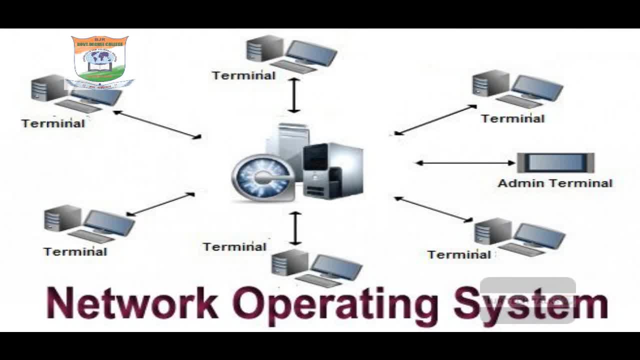 message, passing between the different process working in different systems. so, friends, these are the things we need to know about the distributed systems. so what do you mean by distributed system? if you have an operating system which supports, if you have an operating system which supports the network, then call it as the network operating. 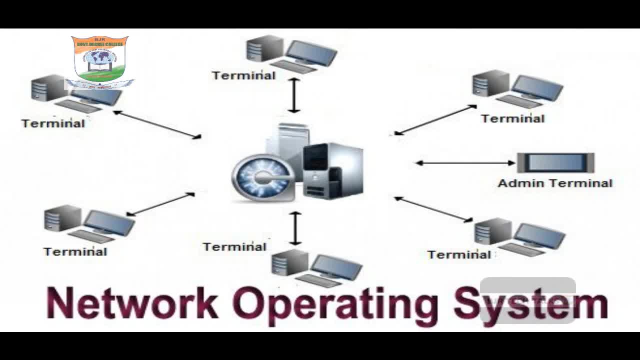 system and if you have a network or if you have a network in which all the computers or all the systems which are interconnected, and even though they are located physically far, but they are interconnected, accessing some shared data, then you call it as the distributed system. and in this distributed system you have, we have learned about certain definitions like a network. 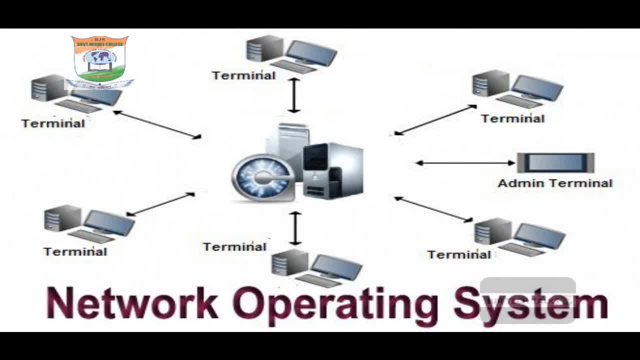 and a kind of networks like lan man and van. and also we understood that there is a special operating system called the network operating system which can do the file sharing, the communication and the message passing or message switching or message exchanging, etc. so let's move on to understood, to 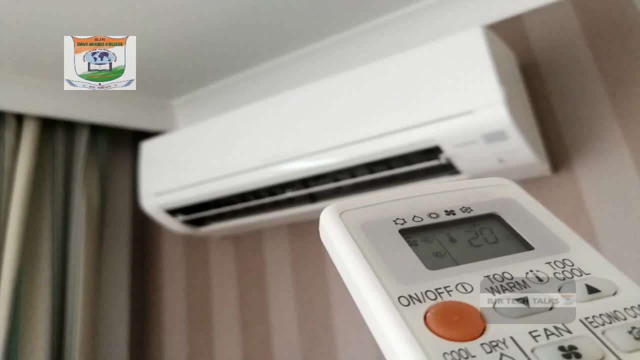 know about this special purpose systems. Let us try to observe some of the electronic systems in our home If you try to work with, if you try to switch on, use AC, that means the air conditioning unit. So that means you are switching on with your remote and the AC is getting powered on. AC is working okay. 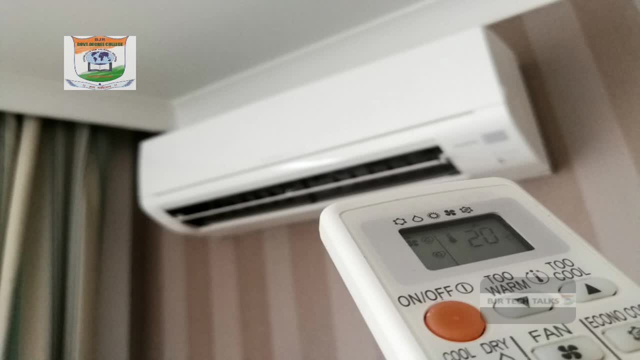 And when you- I mean when you finish- you can switch it off. That means you are saying something to the AC or the air conditioning unit and air conditioning unit is responsive for your request and it is doing some job. So that means that means air conditioning unit is having a CPU correct or not, right? 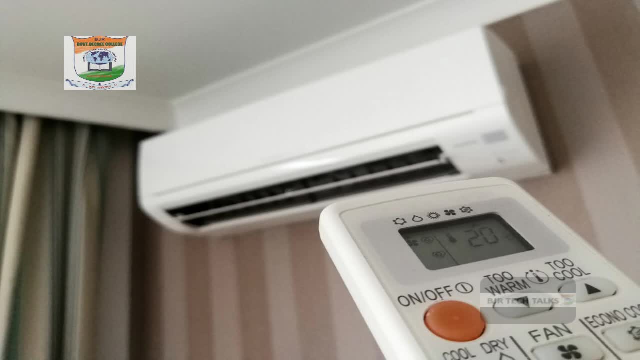 At the same time, air conditioning unit is trying to understand what you are saying. right, That means air conditioning unit is also having an operating system, Because without operating system, without operating system, any system cannot be responded to the user right. 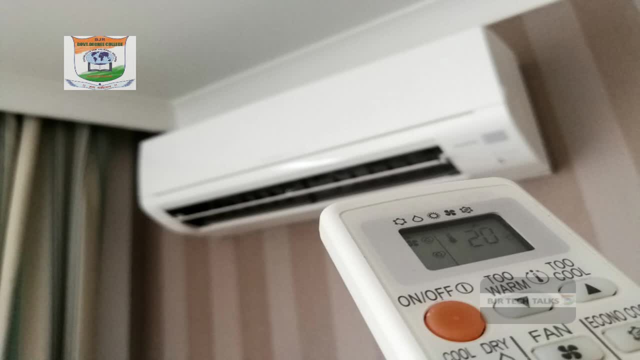 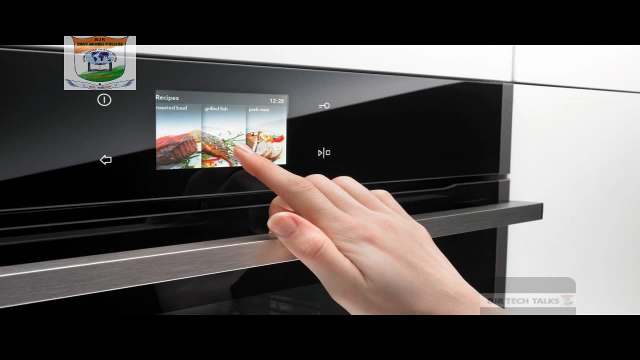 So now the same case with the microwave oven also. So if you say that to cook particular item, so microwave oven will do that. If you say stop, it will stop. So that means even microwave oven is also having an operating system. 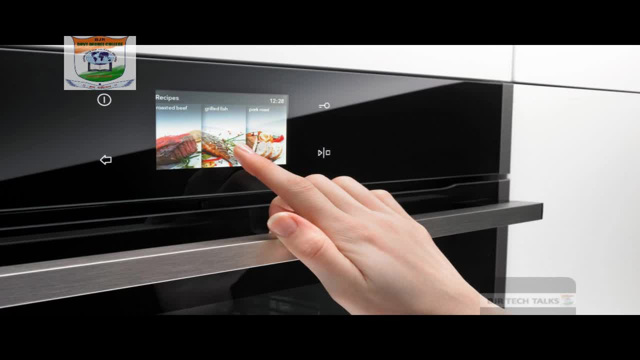 At the same time, it is also. But what is the difference between the traditional operating system which is running in our computer and the operating system which is running in the air conditioning unit or the microwave oven? Friends, this is a special kind of operating system and since it is doing very limited operations, since this operating system is doing very limited operations and it does not require huge amount of space, 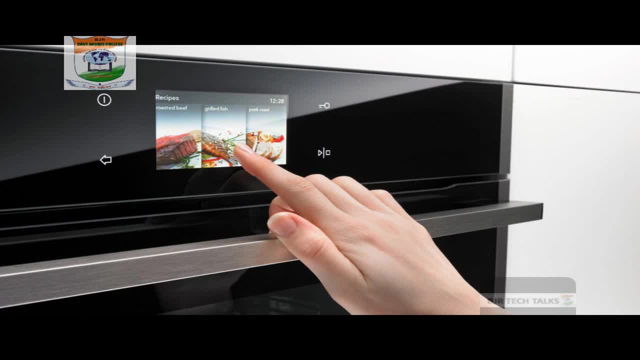 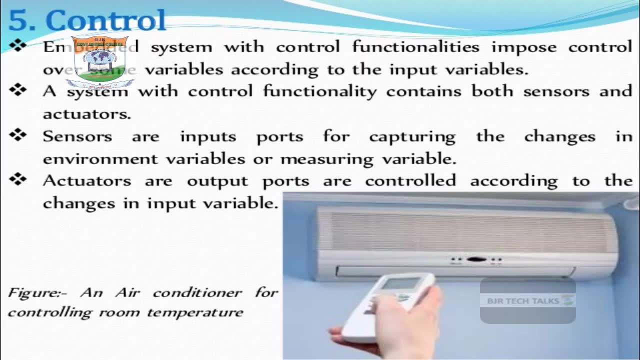 So what they try to do? They try to make this operating system into set of instructions, and these instructions are being embedded: E-M-B-E-D-D-E-D. These instructions are being embedded in a small chip- okay, And this chip will be associated with the air conditioning unit or will be associated with the microwave oven or any other electronic instrument. 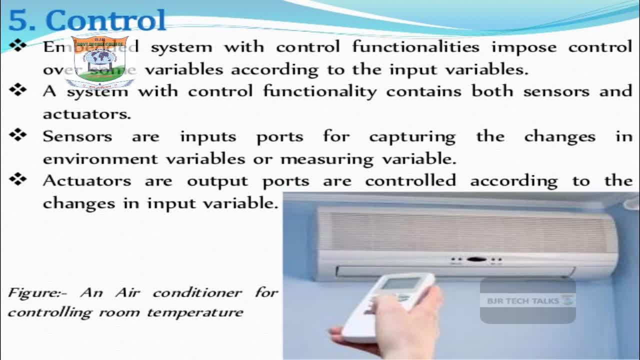 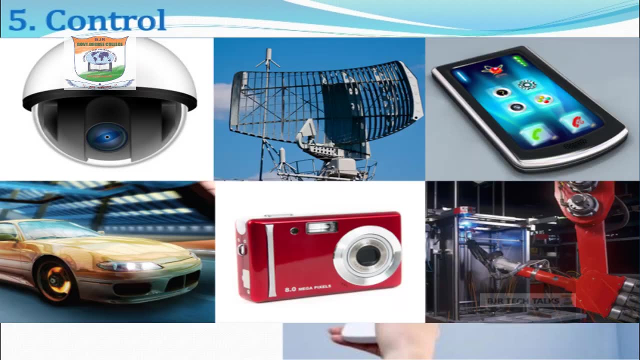 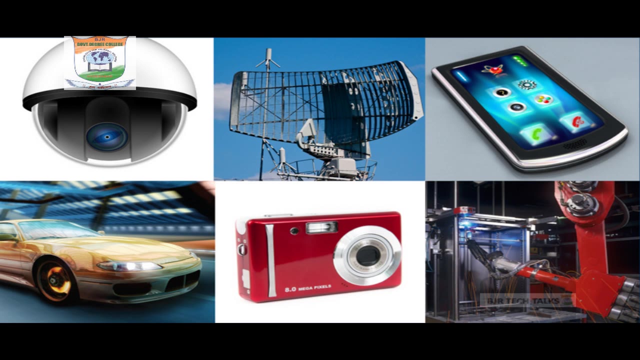 Or any other electronic appliances. So don't assume that every electronic device will have the same kind of operating system. So the operating system will be differing according to the application or according to the its purpose. If you are working with an air conditioning unit, of course it is having an operating system. 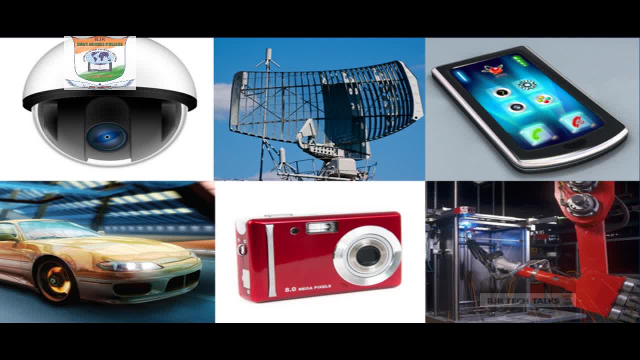 So don't be confused. It is having operating system, But it is Functionality is limited when compared to a traditional operating system. So such kind of operating systems or such kind of systems are called the real-time systems, or such kind of systems are called real-time embedded systems. 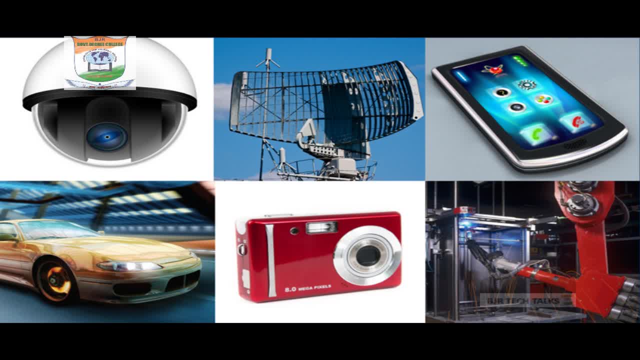 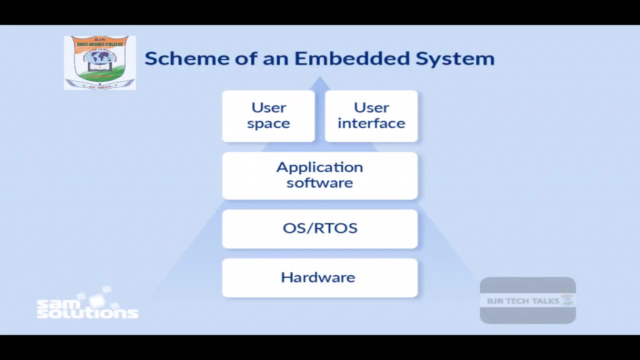 Where here the operating system is not taking a major role, or operating system is not taking a big job, Rather, it is having some predefined set of functionalities And these operating systems are not- I mean- explicitly called for or not explicitly been made used- accessed. 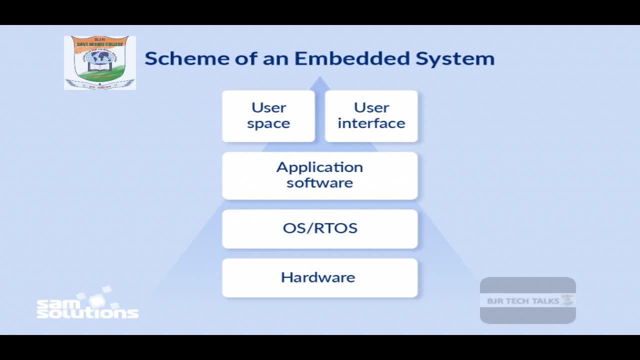 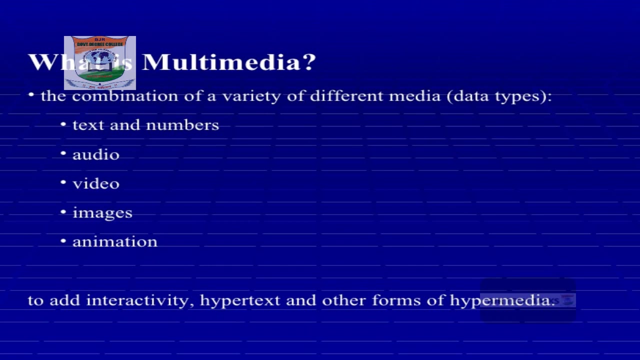 Rather they have been embedded or they have been associated with the hardware chip, So that's why we have to call them as the real-time embedded systems And friends, some of our students and some of our friends. they used to work more with the videos and audios and image files. 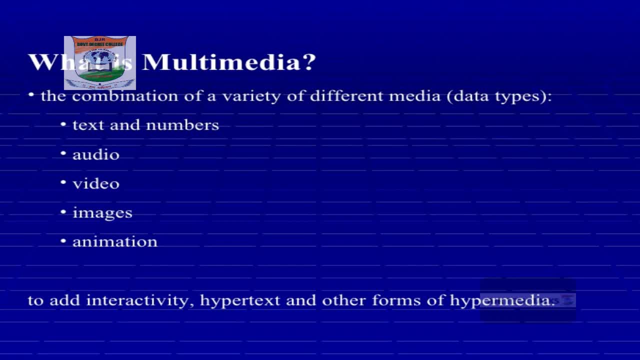 They try to work with some kind of Software, something like we call them as the multimedia- So that means multimedia systems- which tries to overlap with the videos, joining the audio with the video, and they work with the frame rate, the pixel rate. 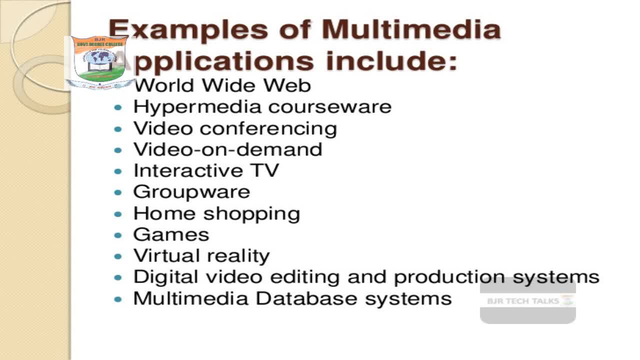 They might be working with MP3, MP4, DVD kind, the video conferencing some they might be working with the video clips. So such kind of system is called the multimedia system And Such systems will have a different kind of operating systems. 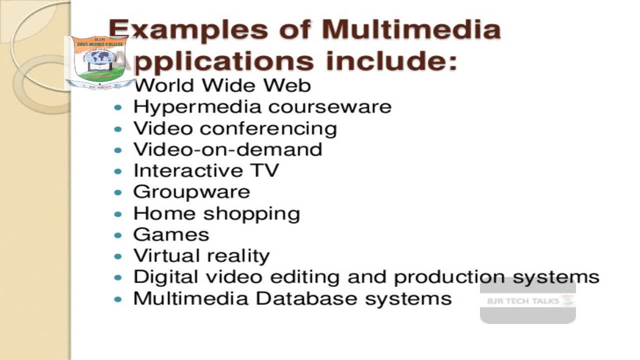 Of course such kind of systems will also have, will also be working with the traditional operating system. but the traditional operating system can be a little bit more extended because these systems they work more with the graphics kind And these systems will be more working with the kind of the certain streaming issues like the frames per second, might be 30 frames per second or 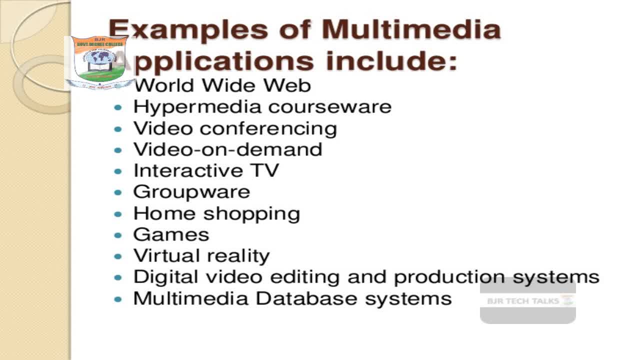 100 frame frames per second, like that. So such kind of systems are mainly supported to work with the gaming kind or the multimedia kind. So these type of systems are called the multimedia systems in which we work with the MP3, MP4, DVD. 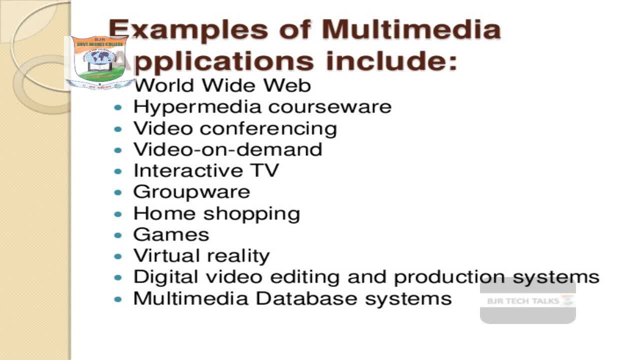 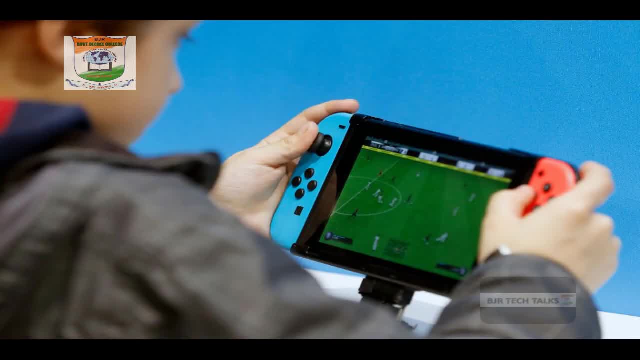 You can work with the video, short video clips, FLV, etc. So, moving on to the third kind, that is, the handheld system. So what do you mean by handheld system? See, friends, the systems which we are working in our hands is called the handheld system. 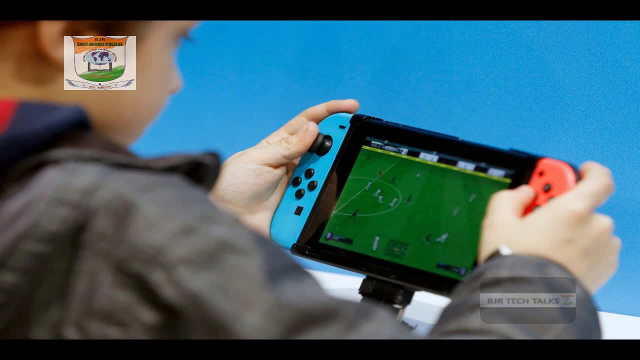 That means the mobile phone or the tablet we are using. It is the best example for the handheld system. So can you say what is the operating system it is having? Yes, it is having the operating system called Android, Okay, And. 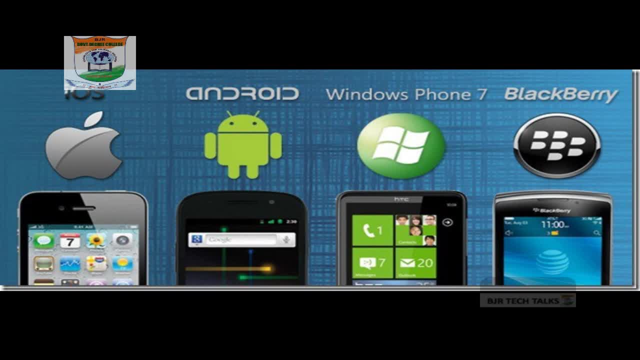 For example, if the computer has been manufactured with the Mobile system, then it is having a specialized operating system called the iOS, Apple, iOS. So iOS is a commercial operating system, whereas the Android is the open source operating system. So that means even the handheld systems. they have their own operating system, like Android. 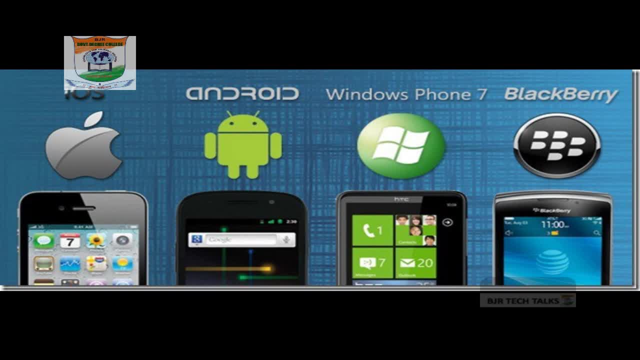 And again the Android. we have different kinds of versions Accordingly to their generations. these versions will work. So what is the speciality Of this handheld systems? we all know the specialty of handheld systems is the screen or the monitor is very small. I mean maximum it is five to seven inches. 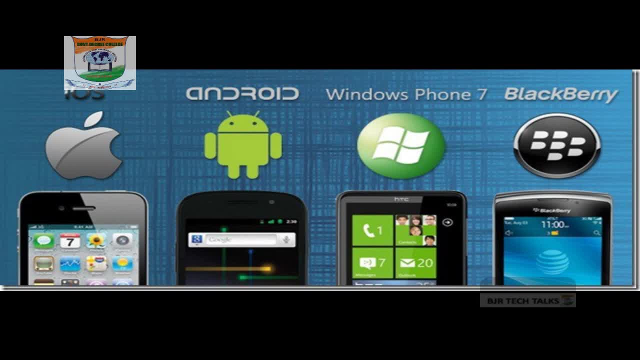 At the same time, these systems can work with the wireless Bluetooth and these systems can work with the wireless LAN or wireless local area network. and they have very other features, like the camera and they have even those. They are confined with very small in size but they can do use computations et cetera. 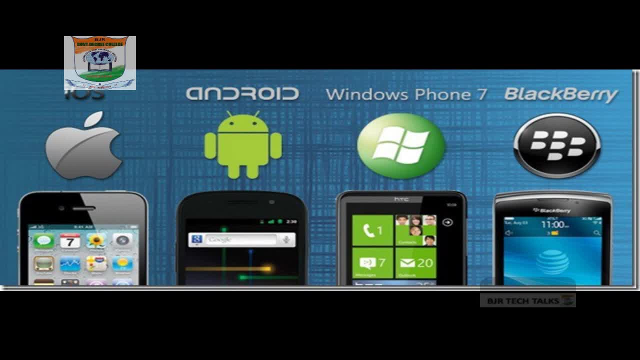 So the operating systems associated with the handheld systems. the operating system associated with the handheld system has a different kind of role. So, friends, in the special purpose systems, we we try to learn about three sub kinds. The first one is the real time embedded systems. 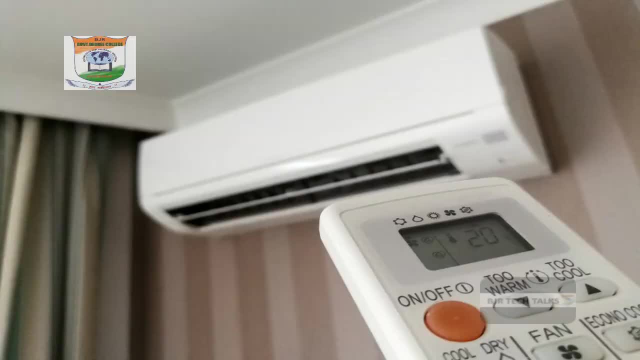 That means, for example, what are? what is the best example we have seen? We have seen the air conditioning. We have seen the unit microwave oven We have. you can also find the operating system, but the uh, the functionality of the operating system is very limited because it has been embedded as an instructions in the hardware chips. 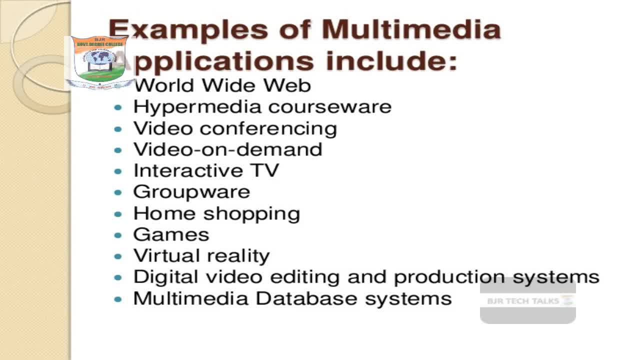 And the second thing, the second sub kind we have seen in the special purposes, the multimedia system, where users at the most work with the uh, work with the photos, videos and audios, Okay. And the third sub kind we have seen is the handheld system. 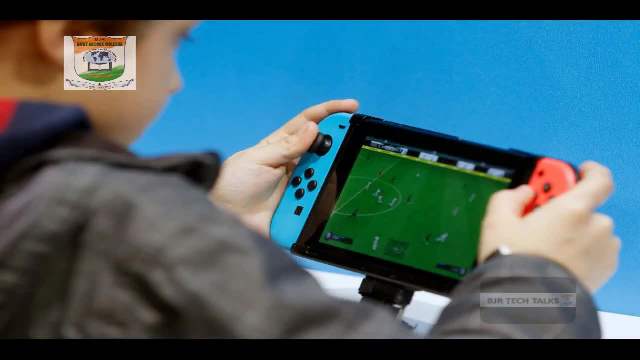 The third sub kind we have seen is the handheld system. And the third sub kind we have seen is the handheld system. Okay, the best example is the mobile phone or the smartphone which is being associated with our hands and it is having a different kind of operating system, like the android operating. 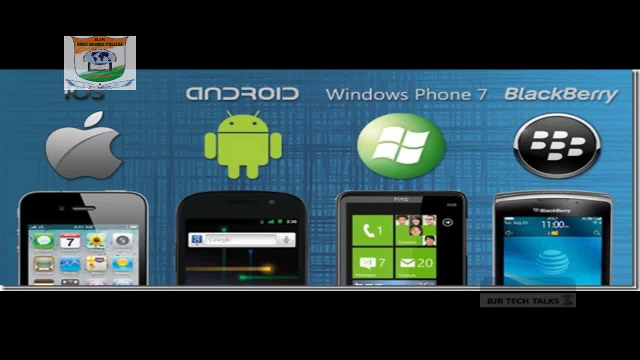 system or the apple ios operating system, and it has its own special functionality. and it has its own special functionality extended with respect to the bluetooth, extended with respect to the wireless lan, and it has its own the cpu. at the same time, it has its own the ram and the. 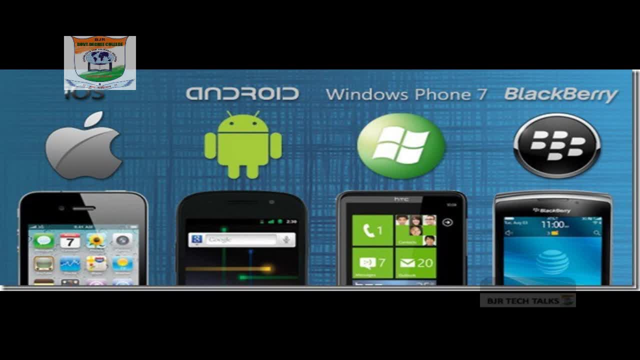 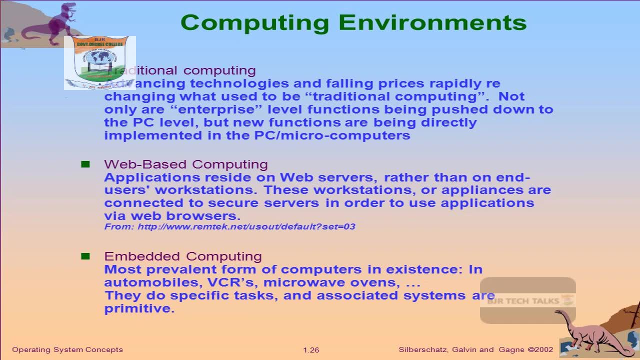 cache memory. so, moving on from this special kind, a special purpose operating systems, next let us try to understand the computing environments. i mean, what are the various computing environments which are available, so that we can be acquainted much more about the operating system? so, in the computing environments, 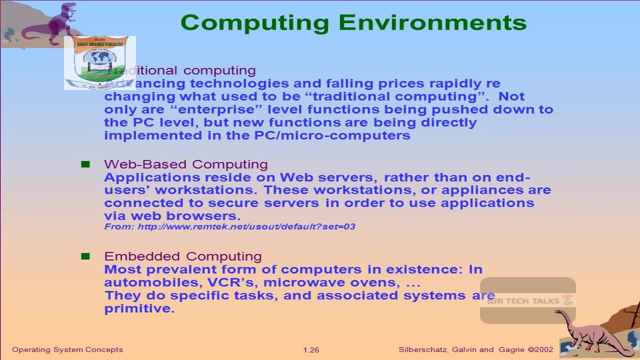 the first environment is the traditional computing. so traditional computing means where you work with a computer, where you work with a laptop. so this is the traditional kind, where you work with a word processor or you working developing a simple program, or you can work with a spreadsheet, or you can work with the microsoft presentation, etc. this is a simple kind. 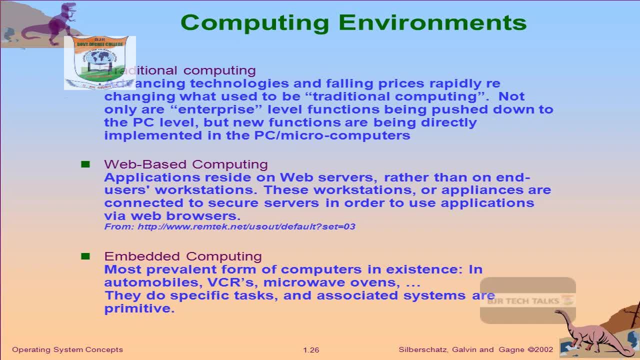 of computing environment. so normally we call it as the traditional computing. if you have your computer running with, if you have your computer running with a simple network, then it is not a standalone computer. then you have to call it as a computer working with a client server environment. see any system which is working within a network and if you find any special any 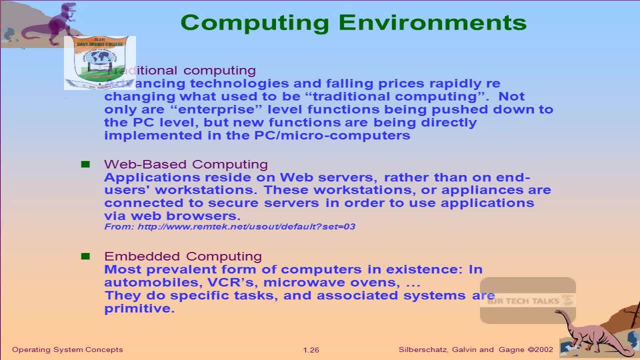 special system which is acting as a server or which is taking the supervisory power and remaining, remaining. all the systems are trying to take the services from the server. then call it as the client server computing. the best example is that the file system. for example, you have a you. 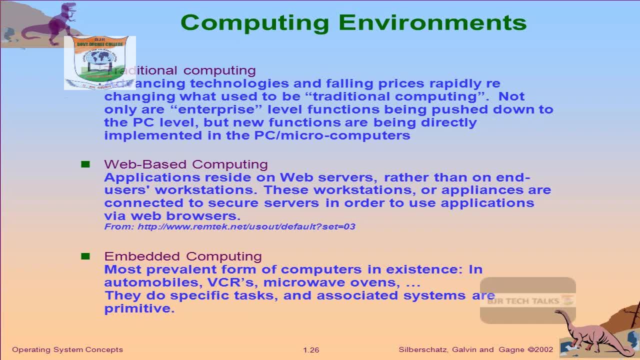 have different kinds of files located at different locations and- and I say that there are different systems which are accessing those files, and I made assume that there is a special kind of system which is trying to monitor all these files and it is taking requests from all the clients or it is taking requests from all the remaining computers. 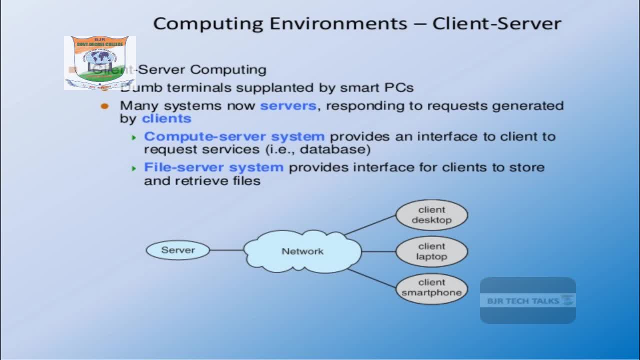 or remaining systems, and it is giving, giving back the data to all the systems. so such kind of environment is called the client server architecture or client server environment. here in this environment you have a network. at the same time you have a specialized system called the server, and server doesn't know how many number of clients are there. server doesn't know which client is going. 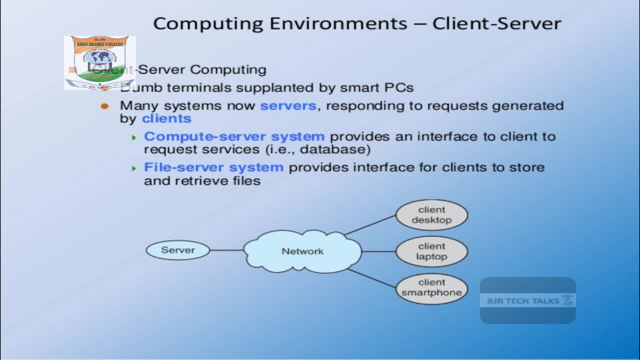 to ask which request, but clients in turn know the server at the same time. clients, every client, has its own request based upon its requirement. so whenever a client, whenever a client made a request to the server, server attends to that request and it tries to give back the service in the form of. 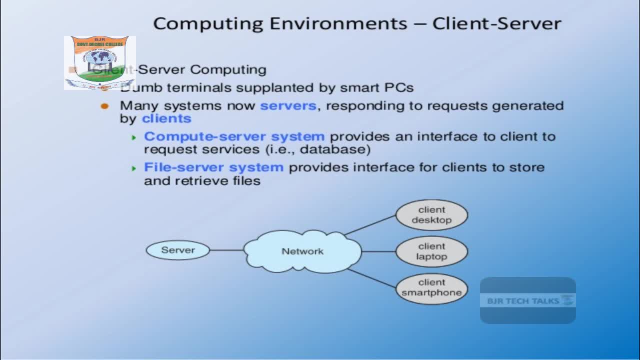 the data, or in the form of a resource, or in the form of Some computation. we have to remember these three points. So when you working with the client server architecture, the client may put some requests to the server and The server may respond in response to the request. 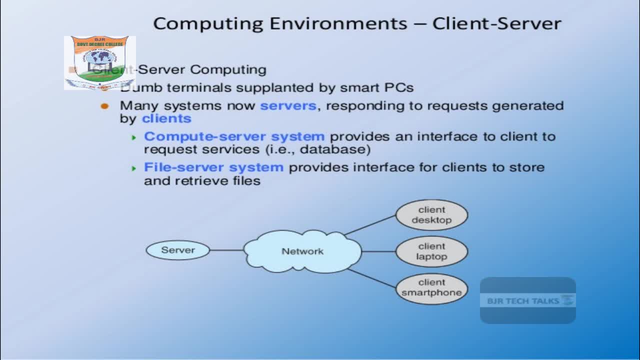 Through it can get back. it can give back a data or it can give back some resource or it can give back some computation also, Probably the server be. the server is having some extra CPU and the client is asking for the remote Accessing. so the server can take the job of this client and it can make it run at the server side and it can give. 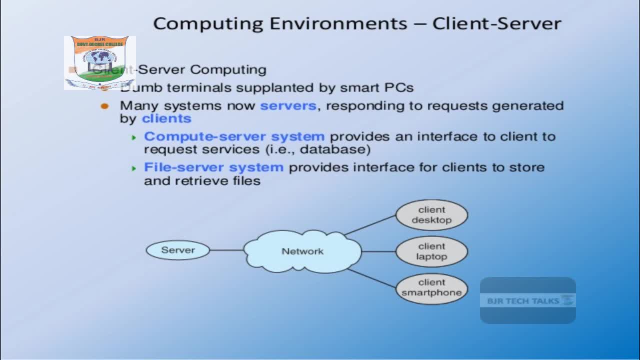 It can give back the result to the client. So this is the second kind of the environment environment that is called the client server environment or client server architecture. the first architecture is the traditional architecture. where there Is no network, the system is accessing. the system is working Standalone manner. in the second architecture you have seen that it is the client server where you have 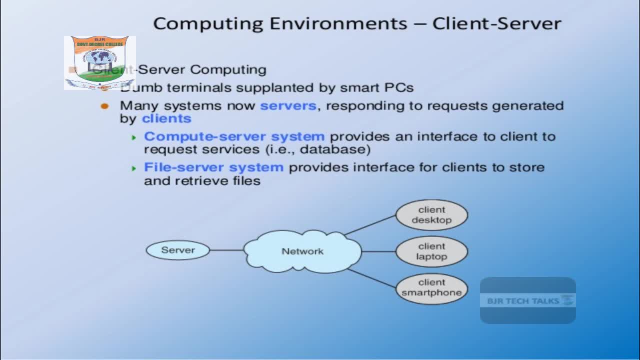 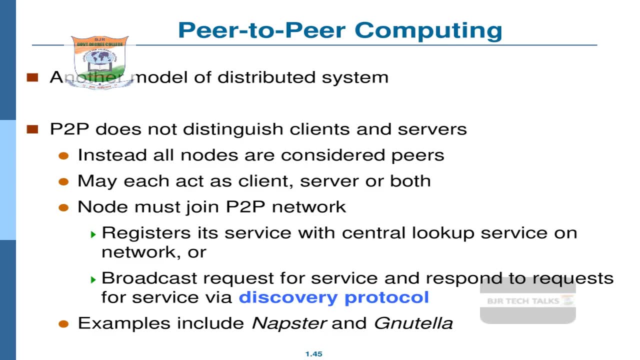 different clients and where you have a few servers which are serving to the Clients. and The third kind of environment is called the peer-to-peer computing. peer-to-peer computing, so Let's try to recall our loosely coupled system Or the distributed couple system. in the distributed system There is no special. 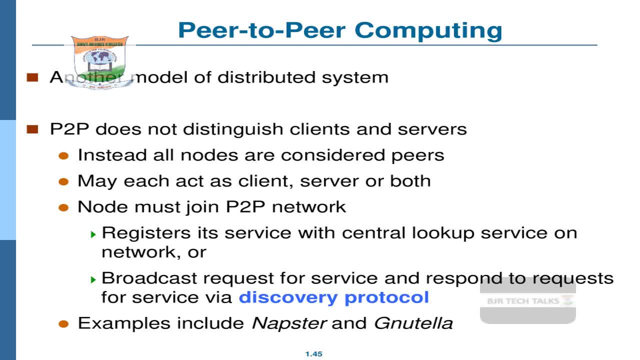 system that is called a server system, in which every system has equal power and every system has its own resources. still, These systems are interconnected through the network and all the systems. they are working in a shareable Resources or they're working with the shared data. So such kind of environment is called the peer-to-peer computing. 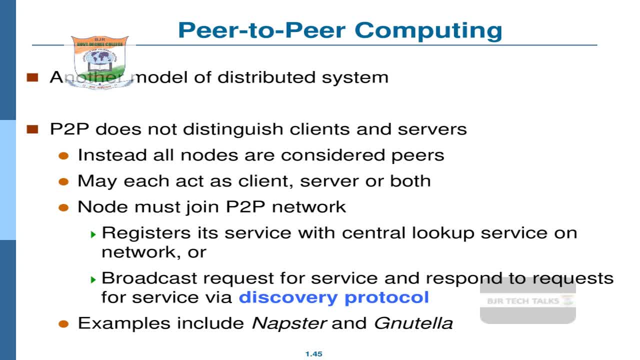 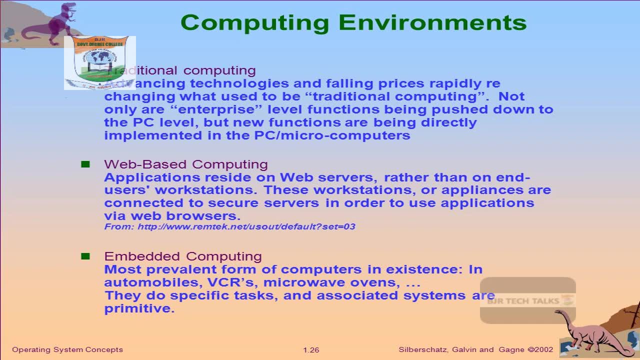 So such kind of environment is called the peer-to-peer computing, Or we can also say it as a distributed system, or we can also say it as the loosely coupled system, Even though the names differ, but the concept remains same. the last kind in this Computing environment is the web-based computing. see up to know what we have seen. 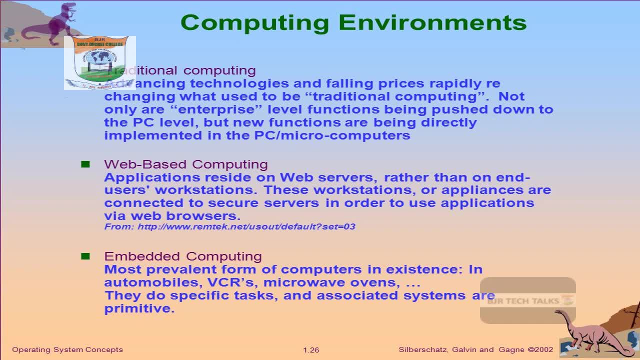 We have seen a traditional environment, the client-server environment. and the third one is the peer-to-peer environment, Or you can also call it as the distributed environment or the loosely coupled system. and the last kind is the web-based computing. so even the web-based computing you try to 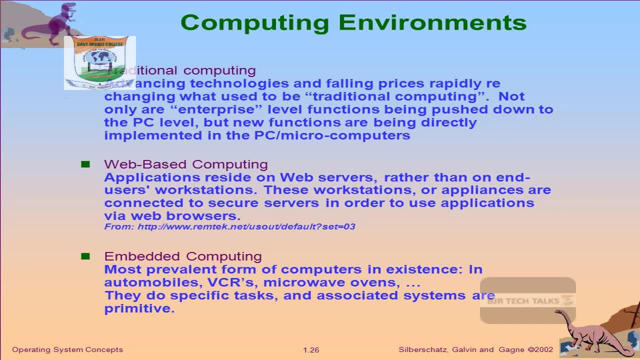 include certain new things like The wide networks or the wireless access. so that means in this, in this Environment, you can see different devices which are working in the network, both in the form of wide, in the form of wireless and at the same time, Basically these kind of systems, they work with the world wide web, So they work with the. 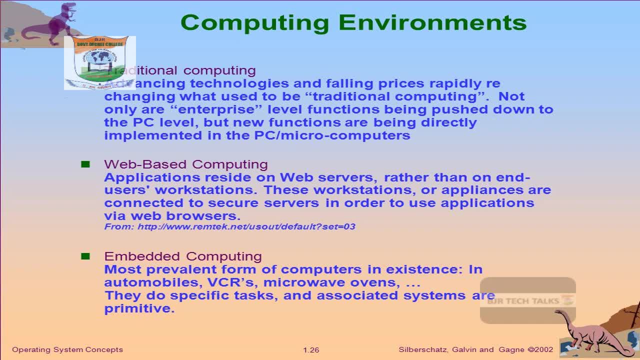 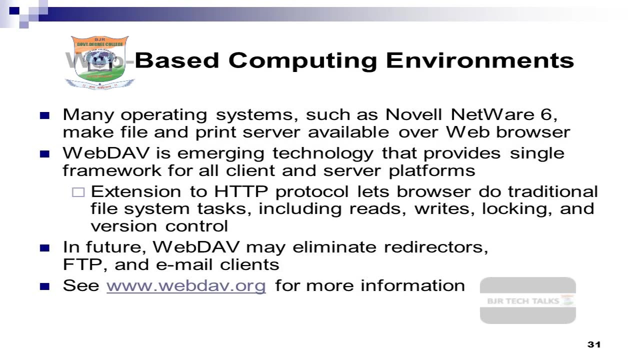 Networking, they work with the world wide web. That means they work with the Internet, So that means they have the faster network connectivity, So provided by the networking technology, or they have the optimized network implementation code either. so these systems, they have a specialized and algorithms called the load balancing, in which 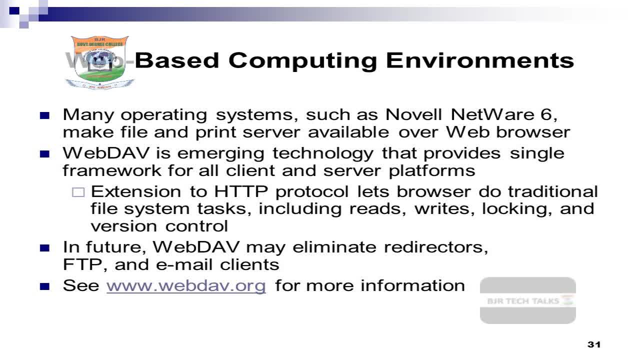 It tries to, it tries to share the load or it tries to balance the load depends upon the request. So this is the fourth kind that is working with the world wide web. that is called the web Environment or web computing environment. So in the environment, what we have seen, the first one is the traditional systems. 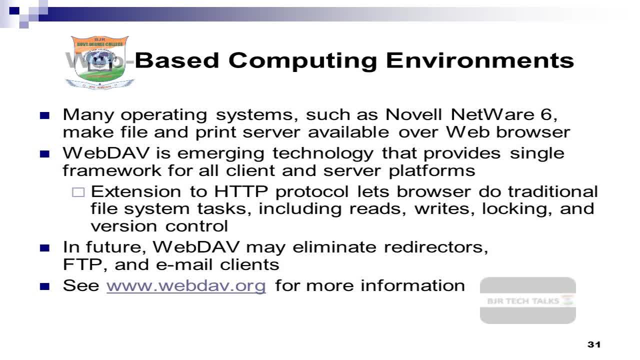 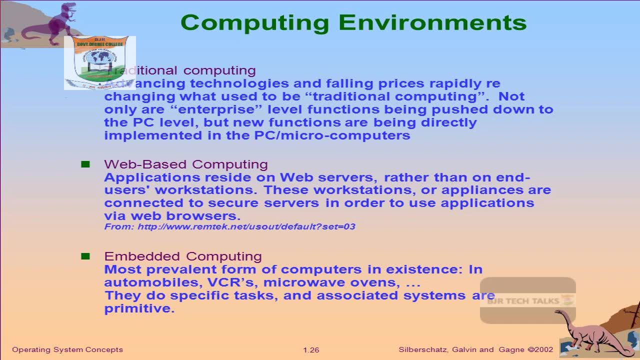 Where it is also called at the standalone systems. and the second one is the clients over architecture and third one is the peer-to-peer. So that means in this architecture we have distributed environment. and the last one is web environment means you're working with the Networking, some kind of wide or wireless. So what is the specialized in this? 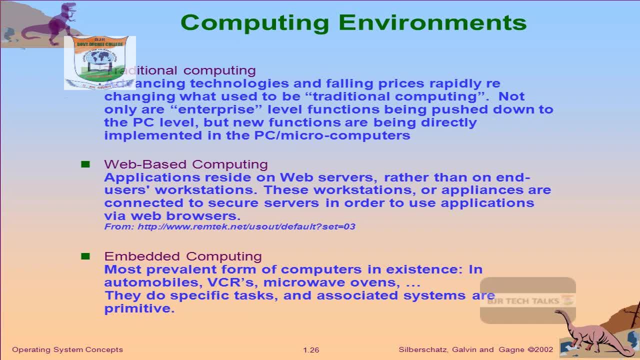 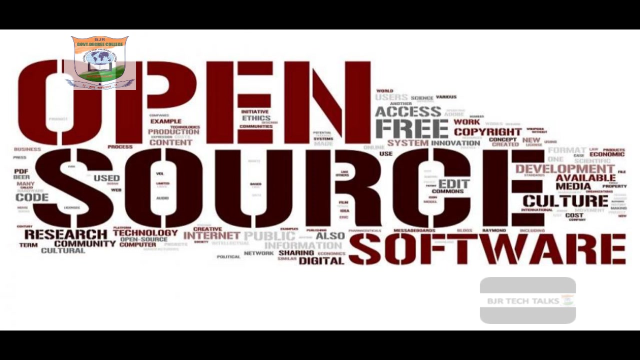 We have the network implementation special technology or the network implementation optimization also. at the same time We can, we can also see about the load balances within the, this kind of network or this is kind of environment friends. for every Commercial system there is an equal, open system. You can make a point of this statement, what I am saying for every commercial system. 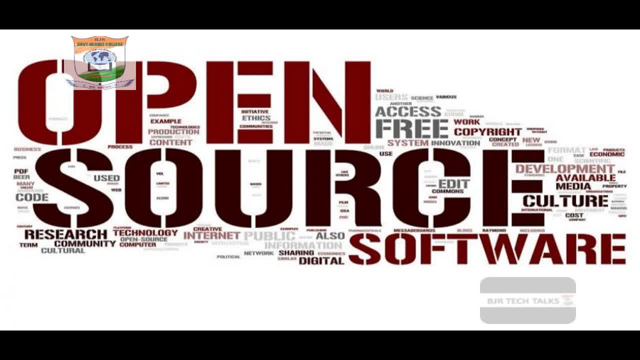 You can. you can have an equal performant, equal perform or equal functionality Associated open system. So what do you mean by open system? Open system means it is a system which is freely available and which can be accessed by anyone, and It is not a commercial one. 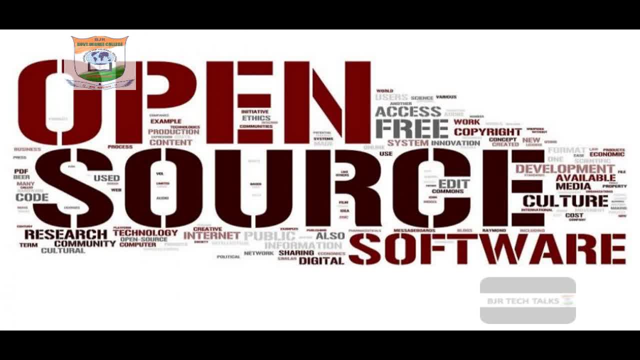 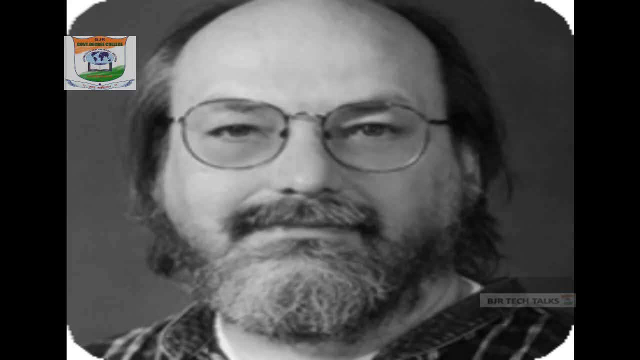 So let us try to understand about this open source operating systems. see, It's very important to recall the efforts of Ken Thompson. So Ken Thompson is one of the person, one of the greatest scientists in computer science domain. He has developed the unix operating system and Unix operating system. my dear friends, 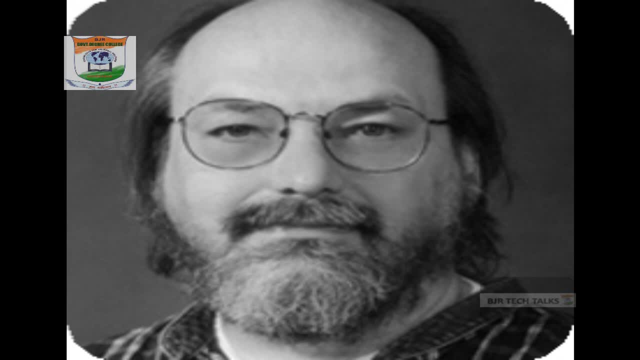 it is not a commercial operating system, rather it is an open source operating system and the ken thompson sir, can the great ken thompson, has given the source code for the unix operating system and he has kept that source code over the internet. many software companies they have copied. 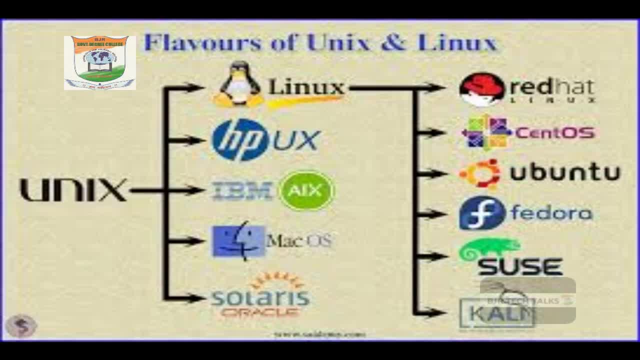 that source code and they have modified. they try to understand what exactly the operating system is working and they can easily modify that source code and these software companies. they mounted these source codes into their own operating systems and they have called, they have name coined different, different kinds like the bsd you, bsd, unix or 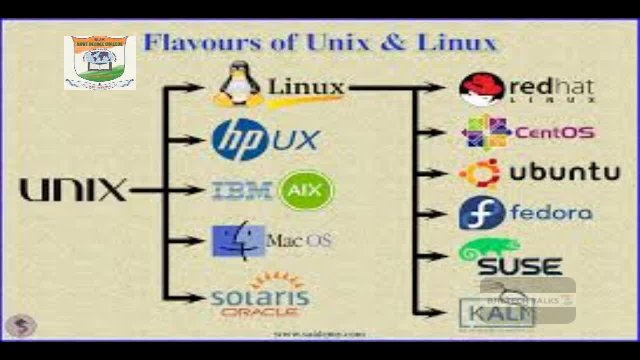 you can have different names for different unix versions or different flavors, or and after that, this unix operating system has been refined much more to make it graphical user interface, called it as linux. so linux is an extension for the unix, okay, and linux is much more of graphical user interface, whereas unix is commanded command user interface. or. 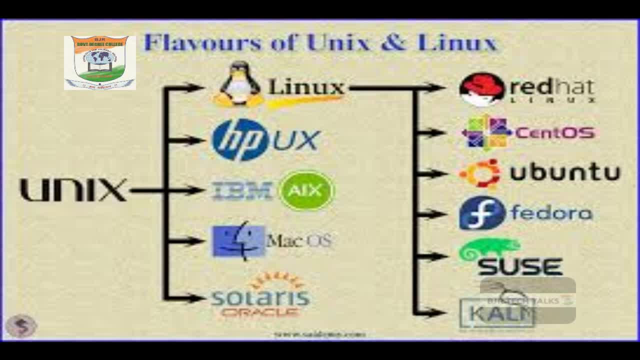 command prompt based, so mostly in the unix, you need to provide the input in the form of commands where, uh, the linux is an operating system which is competing the microsoft windows and apple, uh ios, uh, apple ios operating systems, and it is a parallel system. it is a parallel operating system. 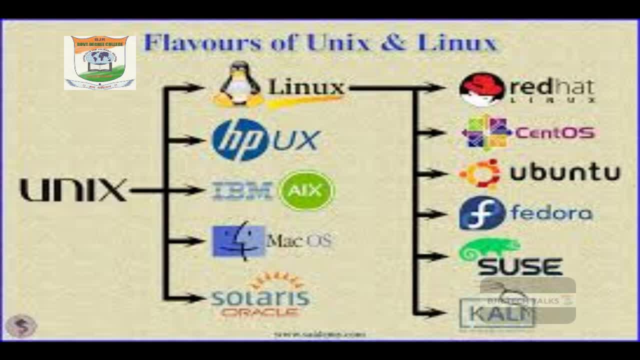 which is working with the was working with the same functionality. probably it is having much more functionality and it is something like having this graphics user interface again in the linux. you can see that this is the unix operating system, where the linux is an operating system since linux or again in the linux. it has many flavors: uh, like the fedora, like ubuntu, the sussy. 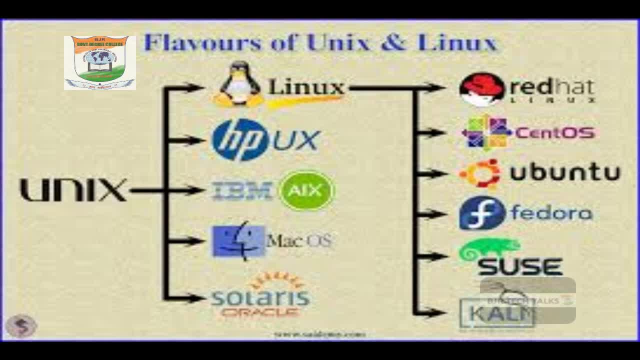 linux, the red hat. linux, this community enterprise operating system. you have different flavors. even the linux has been much more extended to made compatible with the mobile phones or the smartphones, even for the computers also, that, uh, that software. so that operating system is called the android operating system. so 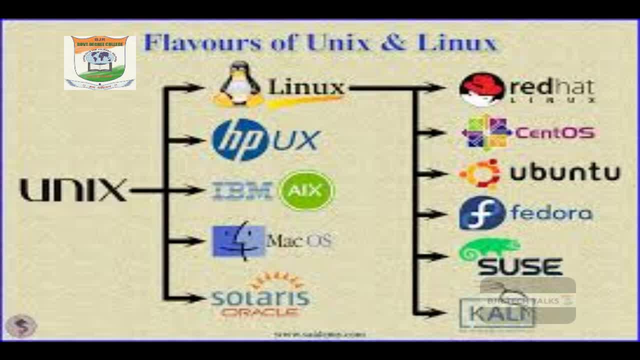 android is an extension of the linux operating system. so this is the basic story behind the open source operating systems. so the basic operating system, the very source, is the unix operating system developed by sir ken thompson. after that the linux operating system has been evolved. after that the android operating system which is right now we are using in our phone. 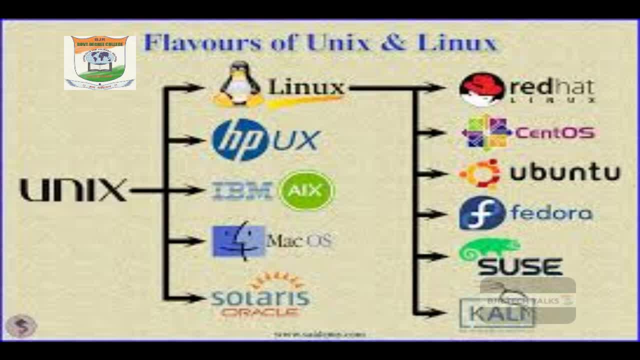 has been evolved. so this is the background story for the open source operating systems. see, the basic advantage of these open source operating systems is that, see, many users or many software companies cannot afford commercial software or commercial systems or commercial operating systems, so they always look for the the second kind, and these second times, like these open 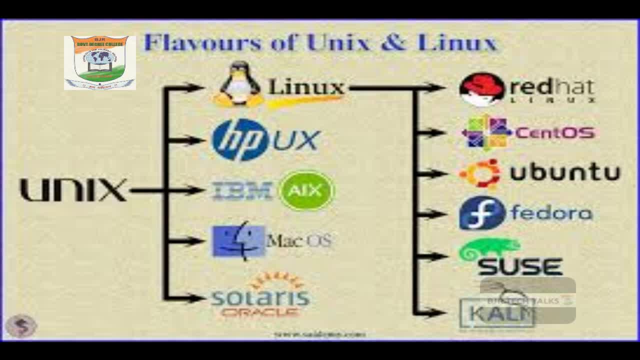 source operating systems, or open source office, always helps uh many users and several users to reduce their cost in development. and you can get a question how these open source systems have been funded. see, several users who are taking the help of these systems can give back a minimal amount of funding to these systems. 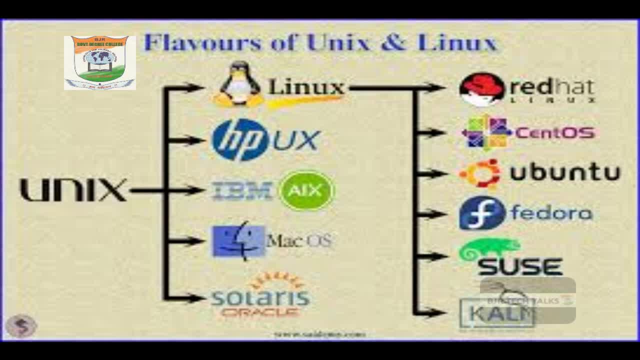 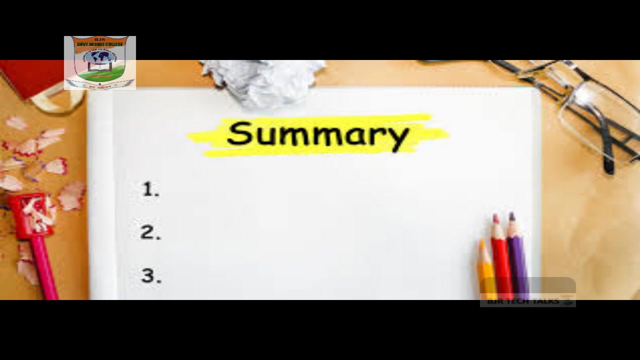 or the to the developers who are associated with the systems and such that they can keep on doing. they can keep on increasing the functionality for those systems. so the revenue can be generated through various support contracts or the sale of hardware or which the software runs right. so that's all, friends. in the today's session we have understood about various environments or